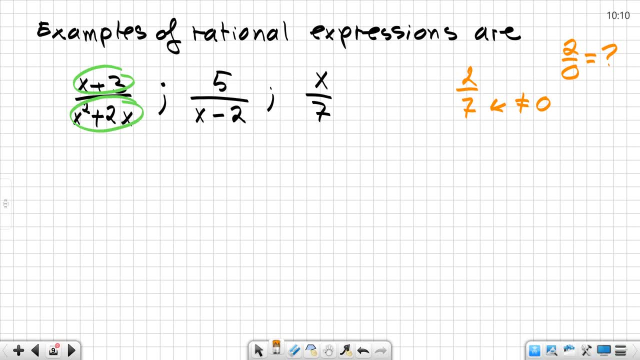 something. This cannot be done. So because we have variables now hiding in our denominator, sometimes there is a chance that you would try to plug in a number in here and that would then turn the denominator into 0. These values have to be accepted. I am not allowed to plug these numbers into these expressions. 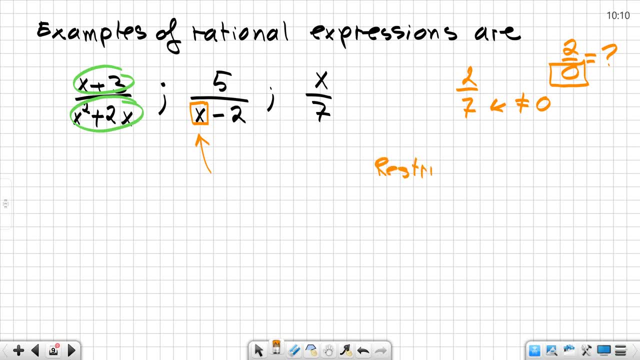 These are called the restrictions. Again, what are restrictions? They are those numbers that, when you would plug them inside, a rational expression would turn the denominator into 0. Now, these numbers are fairly simple to find, In this case the blue one that I have encircled. 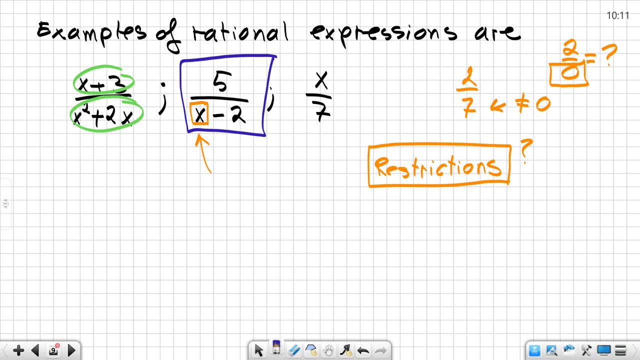 with the square. what number would I not be able to plug into x in this case? Well, in this case I cannot plug in 2, because I would end up with 2 minus 2 in the bottom and 2 minus 2 that would be 0.. 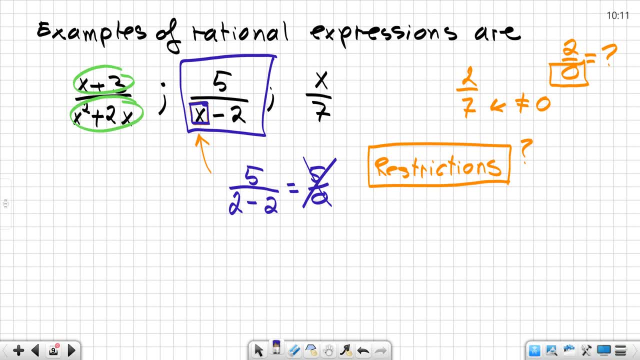 That cannot be done. So how do I find these numbers? I am just going to take my denominators and I will set them equal to 0 and then solve this equation. In this example- the last one- there are no restrictions because there is no x in the bottom. So the first two will. 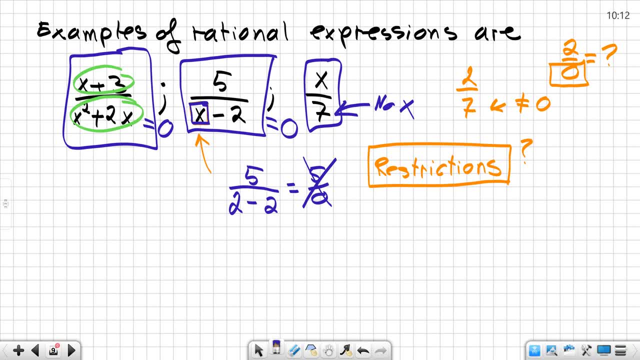 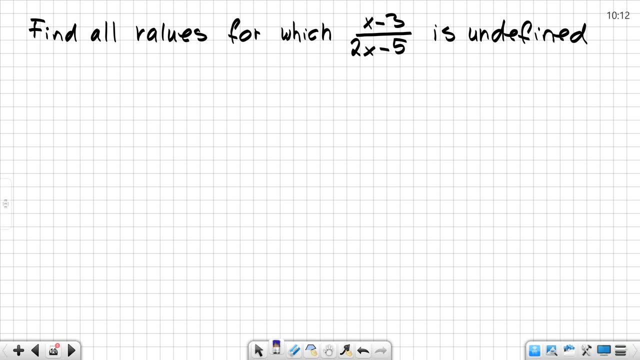 have restrictions, while the last one will not. This will always be the first thing that we are going to find, So here is an example for this: Find all values for which x minus 3 divided by 2, x minus 5 is undefined. 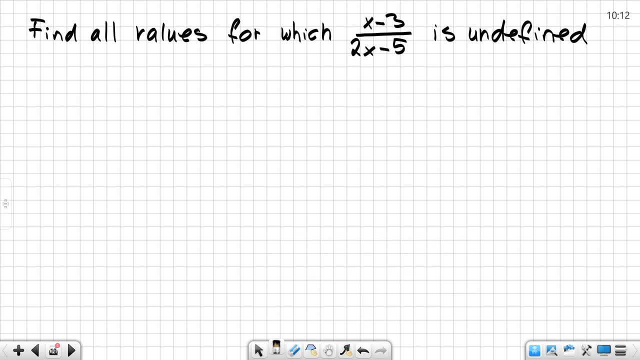 So all I have to do is this. I am just taking my denominator, because there is an x in there, and all I have to do now is x minus 2 times 2, which is equal to 1.. All I have to do now is: 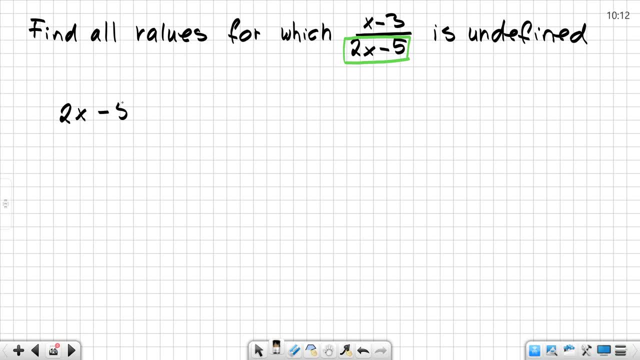 take the denominator and set it equal to zero, solve this equation and those are the numbers that are bad. So the numerator up here that is completely independent from this. the numerator is always good. This stuff in the top: this is allowed to be zero. Remember zero divided. 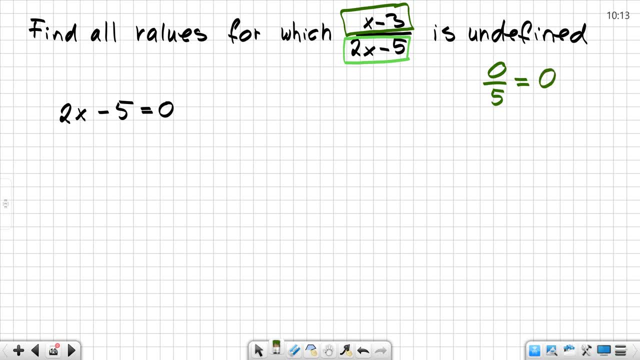 by five, for example, that is defined, this will be zero. So in the top is good, but in the bottom is bad. All right, So let's get to our example here: 2x minus five is equal to zero. The first thing that we are going to do is we are going to add five to. 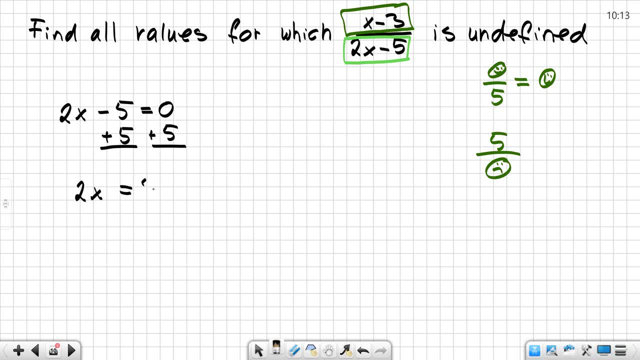 both sides. Now the next step is to divide both sides by two, and I see that five over two is a restriction. That means now I could plug any number into this original example right here. Any number can be plugged in here, But one x cannot be equal to five over two. This was my restriction that I found in my 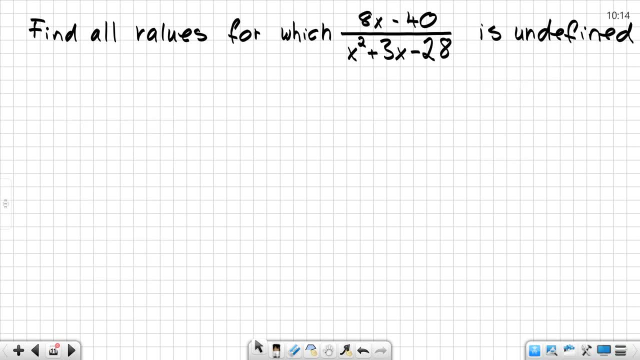 first step. So let's do this one more time. We want to find all values for which eight x minus forty, divided by x squared plus three x minus twenty-eight, is undefined. In short, five over two is a restriction, but we want to find the restricting. So we are going to find the restricting. 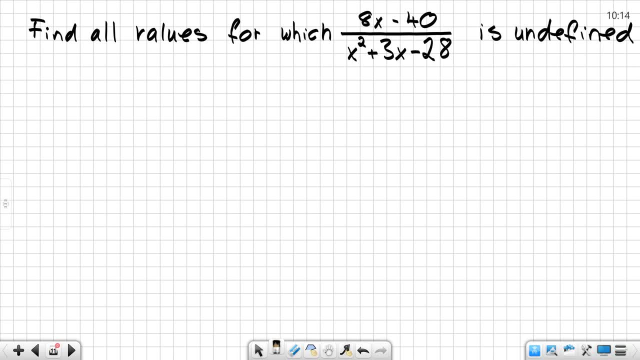 So where are they to be found? Only in the denominator Right. here is where we find these numbers. So all I have to do is I take this and I will set it equal to zero to find the numbers. But because these numbers will turn this into zero, these numbers have to be excluded. 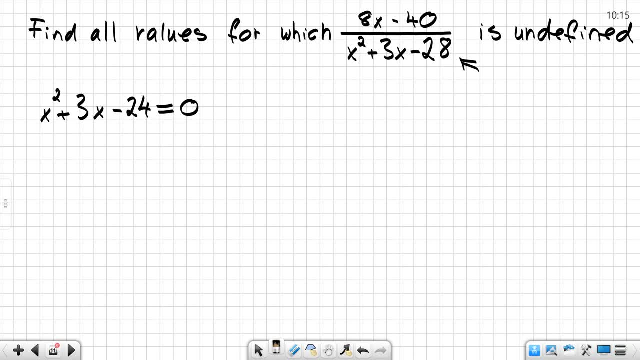 0 to zero, 5 to zero, 5 to zero. excluded therefore, this is this expression undefined. So you remember that we have solved quadratic equations and we do this in this case by factoring. So this is a good, quick reminder and also the reason why we have already solved quadratic. 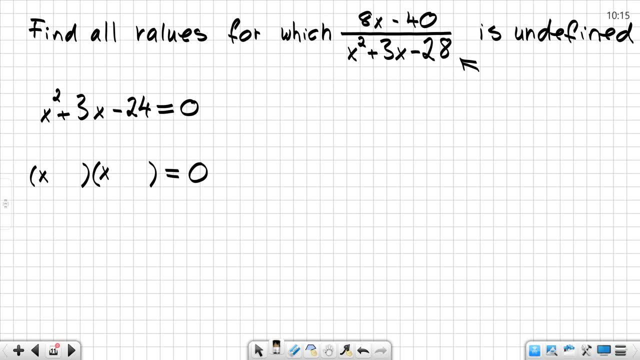 equations. I am looking for two numbers whose product is negative 24, but whose sum is positive 3.. These two numbers would be a negative 4 and a positive 7.. Negative 4 times positive 7 is negative 24.. Negative 4 plus 7 is positive 3.. 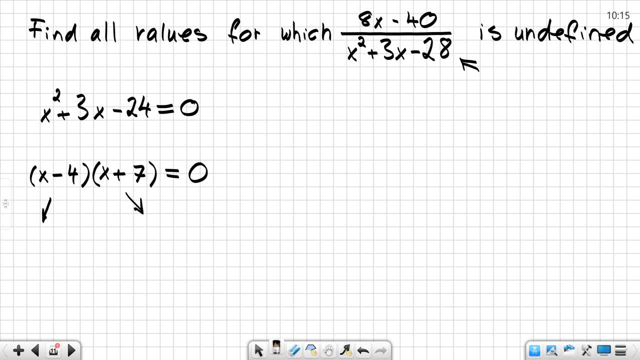 Now we remember that I have factored this. All I have to do is I am setting my factors equal to 0 and solve these two. So I am adding 4 and I am subtracting 7.. That means my restrictions are 4 and negative 7.. 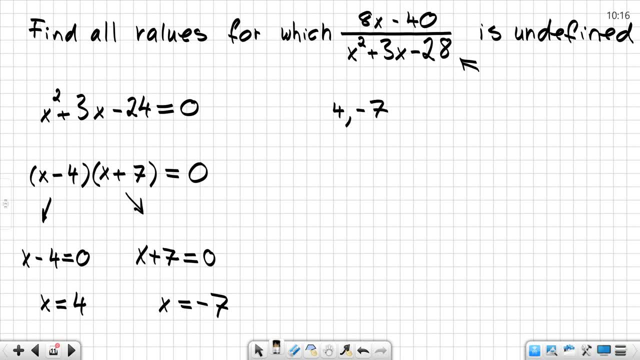 4 and negative 7.. This is what x actually cannot be equal to. I cannot plug in 4 or negative 7.. Okay, since I have done perovski's teachings in the first part, I am none of the outside game. 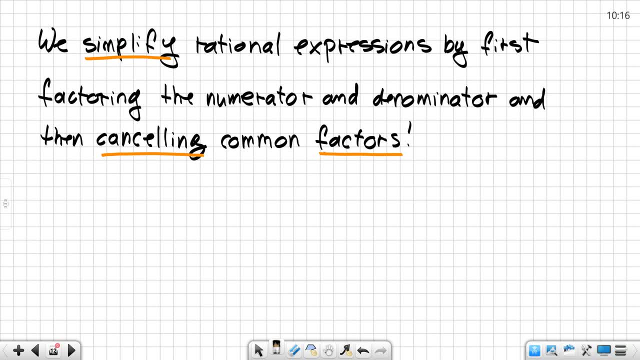 Now let us go ahead a hand and simplify. So what we are doing to simplify rational expressions is factoring everything and then common factors in the numerator and denominator will cancel out. they are giving us examples… attributable, because they will move this forward. 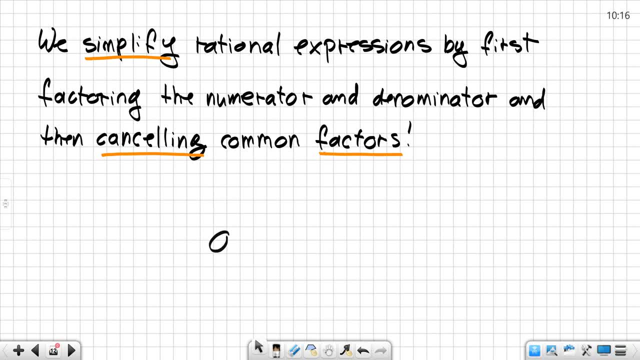 if we have written this method, tell us now what are the correct numbers? The answer is no. about letters, as we always do, I believe. a P over Q if this is a rational expression. times R times R. If R is a common factor in the top and the bottom. 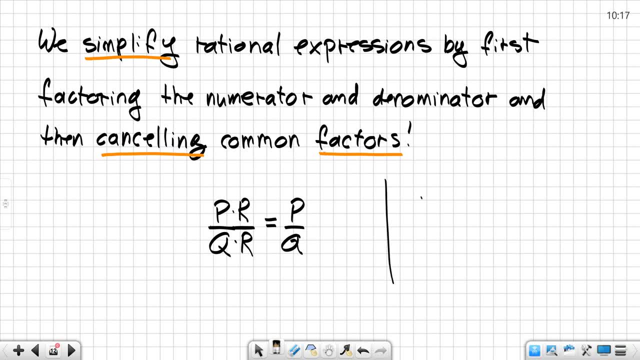 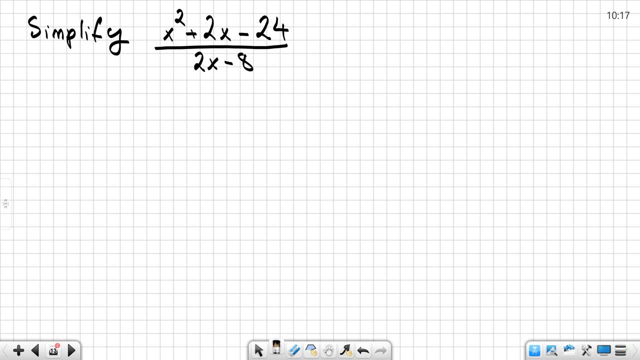 then this can be cancelled out. Remember: 2 times 3 divided by 5 times 3.. This 3 can cancel out and you are left with 2 over 5.. So let's do an example for this. We want to simplify the following rational expression: 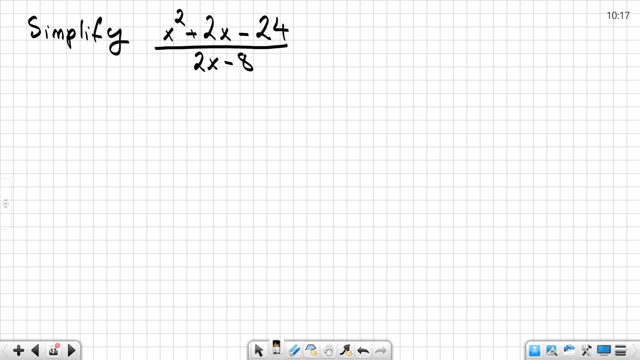 x squared plus 2x minus 24.. So what do we do? You'll see why factoring is going to be the most important part in this section and in the rest of this chapter. We have to know how to factor. I am looking at the numerator. 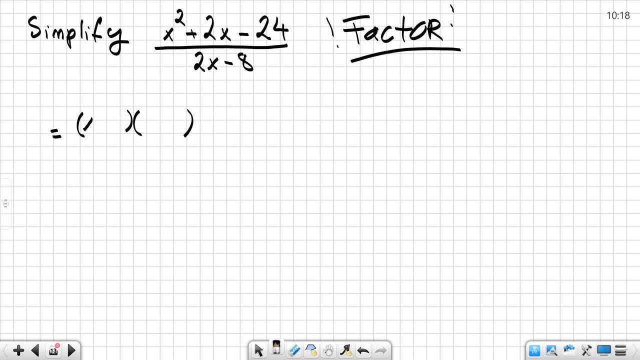 and I know that I can factor this. The faster you are with your factoring, the faster this problem will go: Minus 6 plus 4.. Let's check if this is right. No, this is not quite right. This looks very tempting. 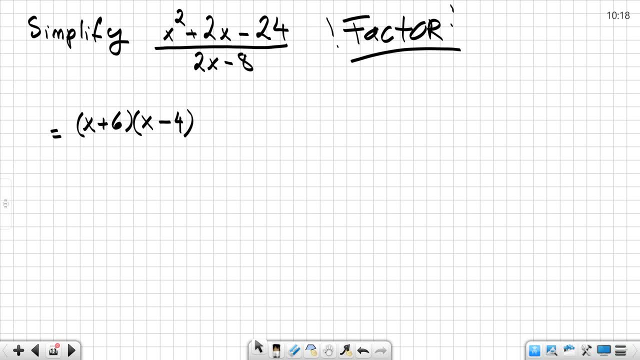 but the 6 has to be positive and the 4. The 4 has to be negative. 6 times negative, 4 is negative, 24.. 6 plus negative 4 is positive, 2.. Now I'm looking at the denominator. 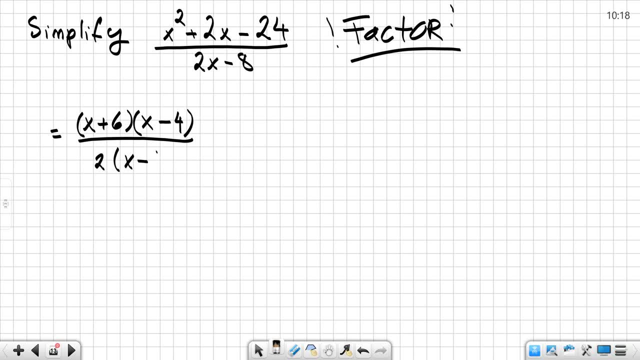 There is a common factor of 2 that I can pull out out of the first and the second term, and I'm left with 2 times x minus 4.. I have not changed anything. This is still the same problem as before. I just put it in the factored form. 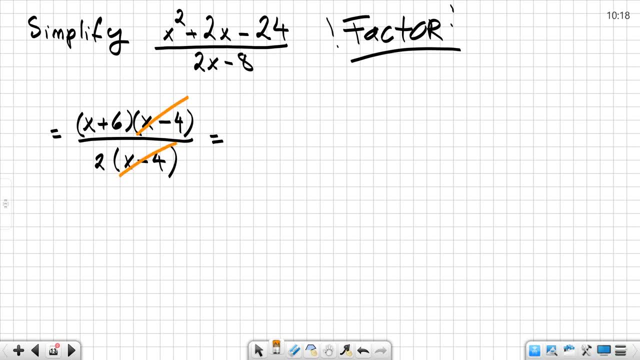 And now what you notice is that there is a factor of x minus 4 in the top and in the bottom, and that means I'm ending up with x plus 6 divided by 2.. The parentheses now in the numerator can disappear. 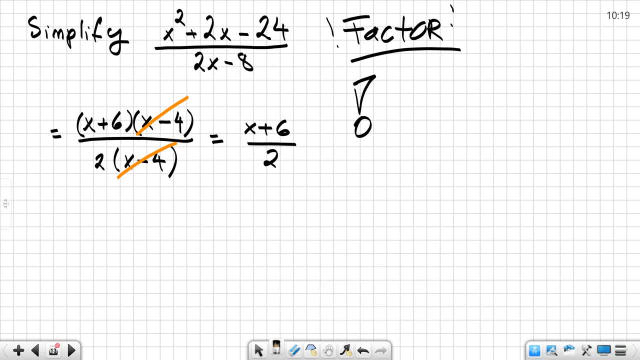 Now be careful. Be careful, Do not do anything with this 6 and this 2.. You cannot cancel out anything, right there? Factors cancel Terms, do not. These are terms. right here? This positive 6 is a term. It is not a factor. 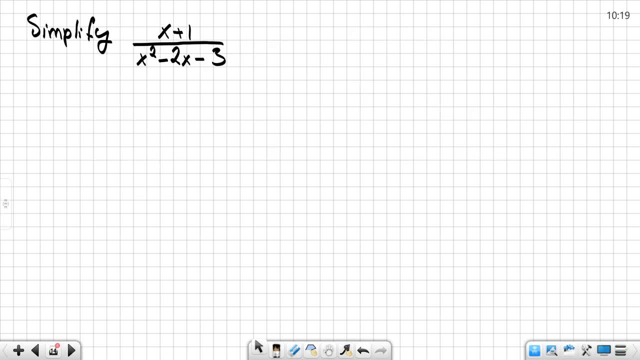 So be careful about this. Let's do one more example: x plus 1 divided by x, squared minus 2x minus 3.. So I'm looking at this and I'm supposed to simplify this: The numerator cannot be factored anymore. 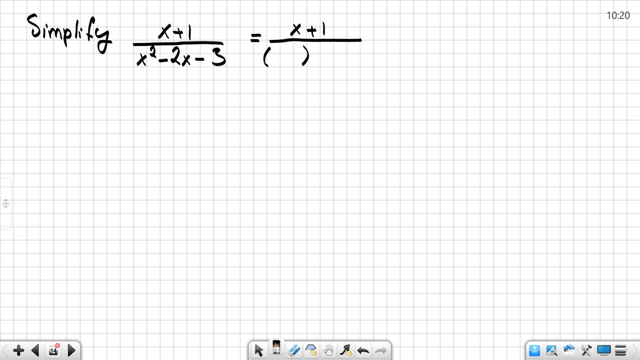 This is what we called prime, But the denominator can be factored. Let's have a look. This should be x plus 1 times x minus 3.. I'm double checking this: Negative 3 times 1 is negative 3.. 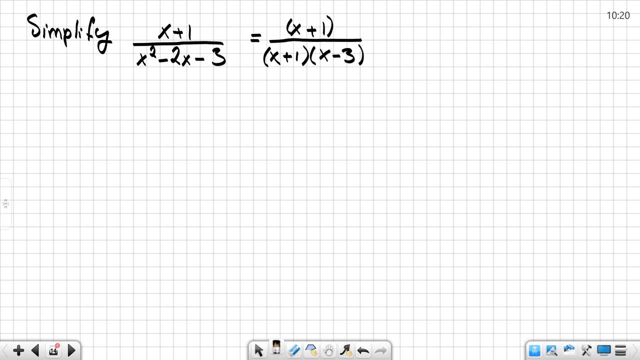 1 minus 3 is negative 2.. All right, Now you can think about. as if this is up there in parentheses, Put a 1 in front of it, if you need to, so that you don't forget something: 1 times x plus 1.. 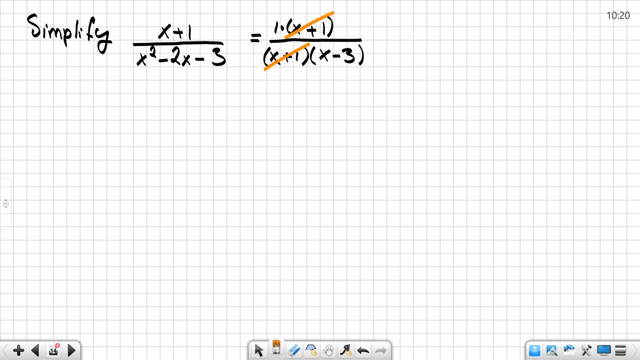 Now the factor of x plus 1 is the one that disappears, and that means I'm left with 1 over x minus 3.. One big mistake is that people are just writing down the answer as x minus 3 because they have factored and they have canceled. 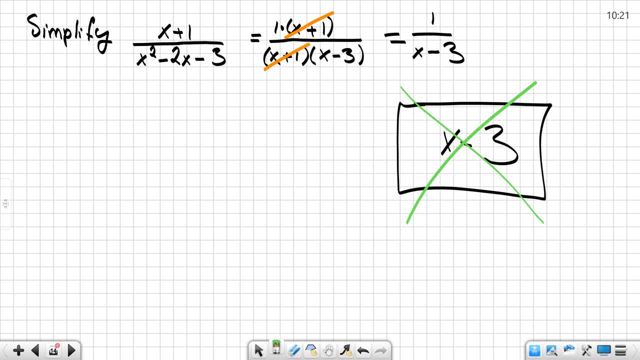 but they do not see that x minus 3 was in the denominator, because it was in the denominator to begin with. Let's do one. I believe this is the last example in this section. One more, All right, We have x squared minus 1 divided by x squared plus 2x. 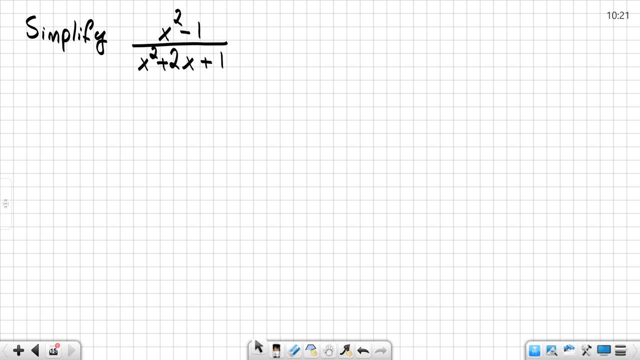 plus 1.. Again, do not cancel out these two things right here: x squared and x squared. You cannot cancel These are terms. What is the first thing that we need to do? Refactor. So I look at the numerator. 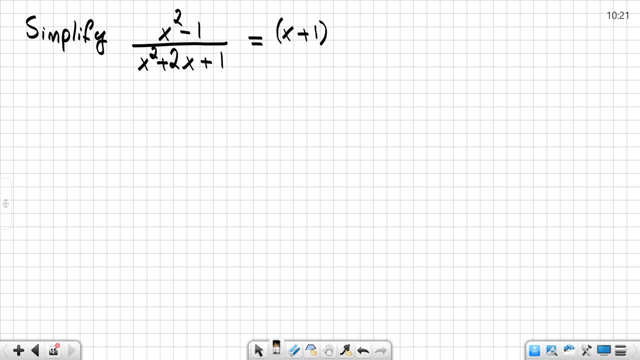 This was the difference of two squares, So this is going to be x plus 1 times x minus 1.. I look at the denominator. This is a trinomial with leading coefficient 1.. And I'm getting x plus 1 times x plus 1.. 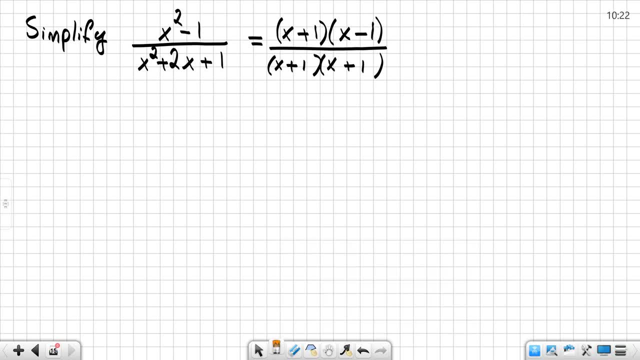 Now I step back from my board and I see that there is a factor of x plus 1 in the top and the bottom That can be canceled out. And now I can drop the parentheses in the numerator and the denominator And I have my answer.